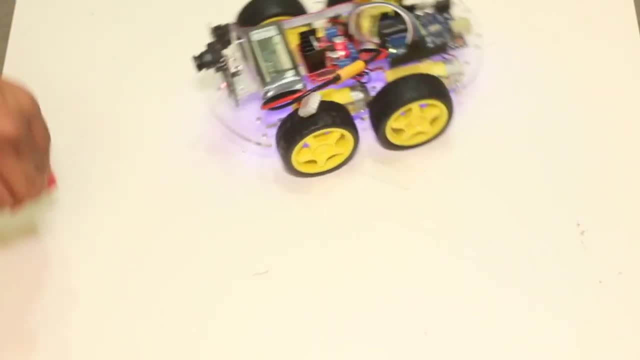 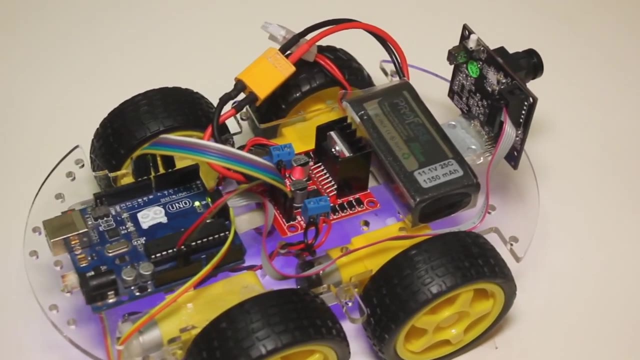 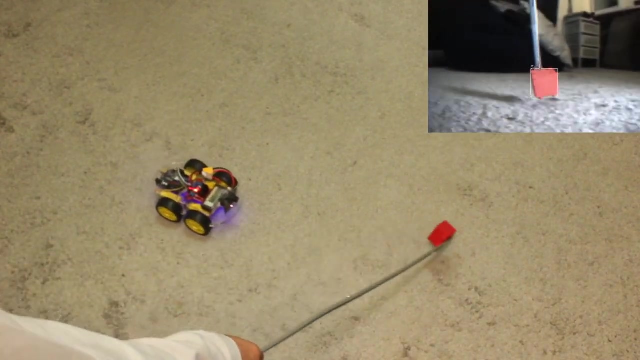 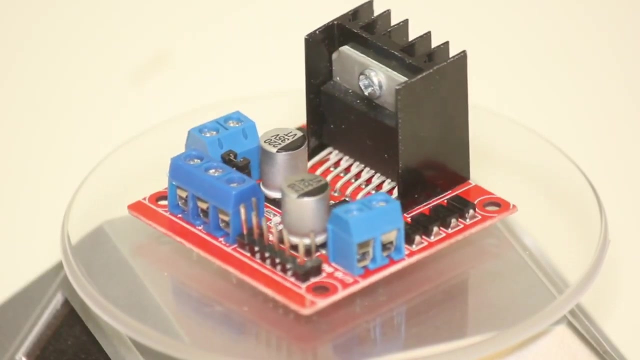 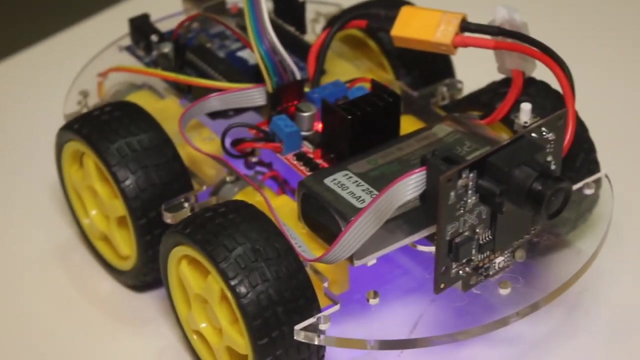 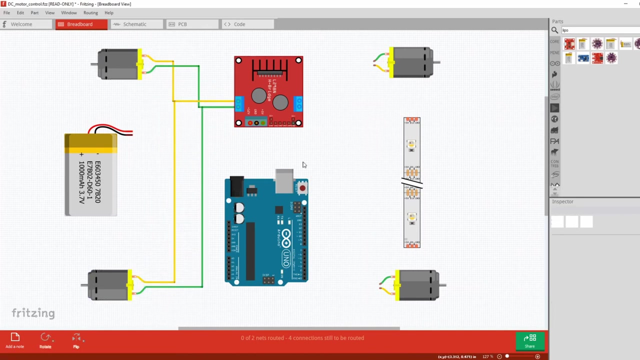 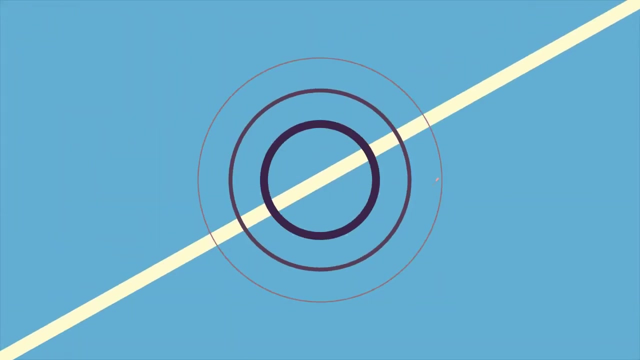 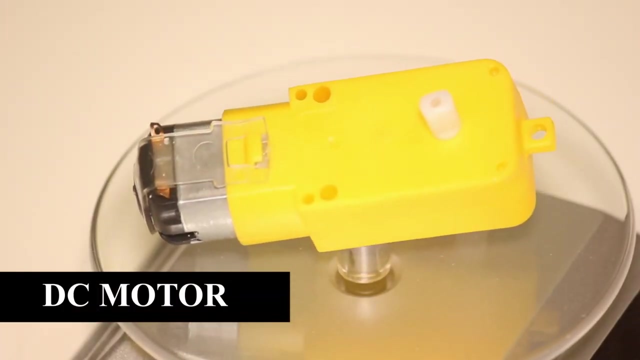 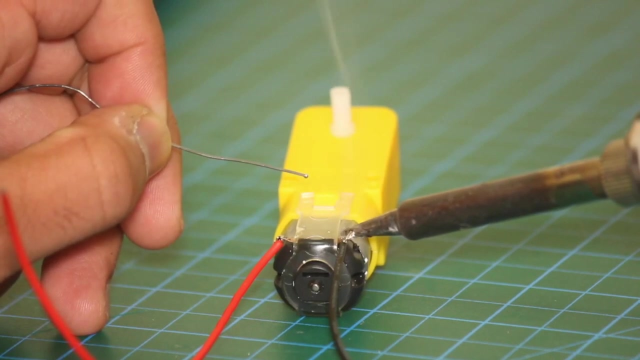 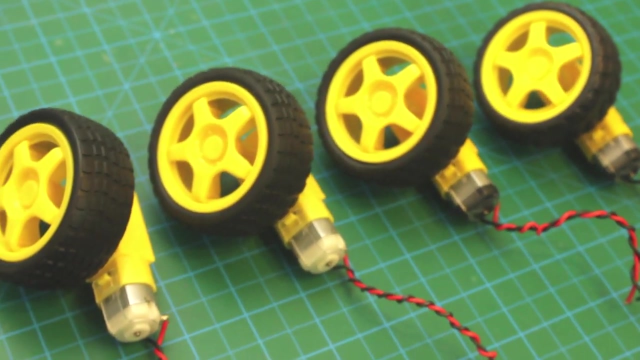 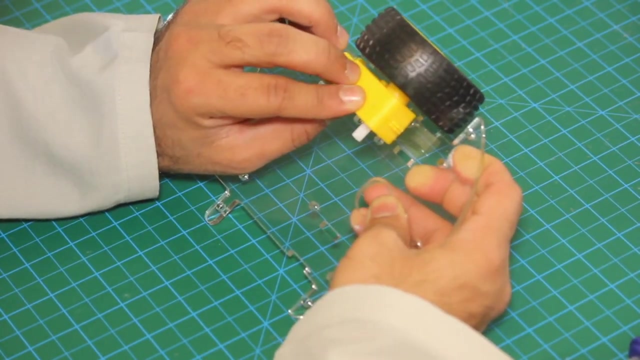 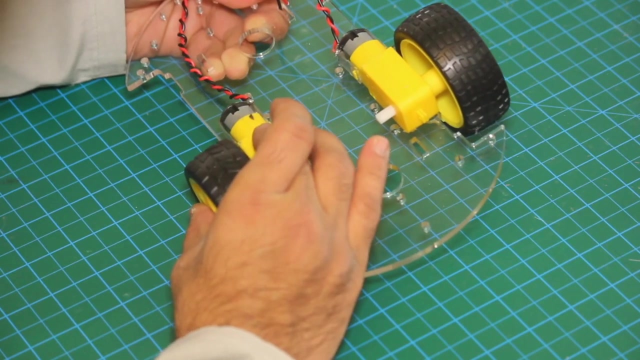 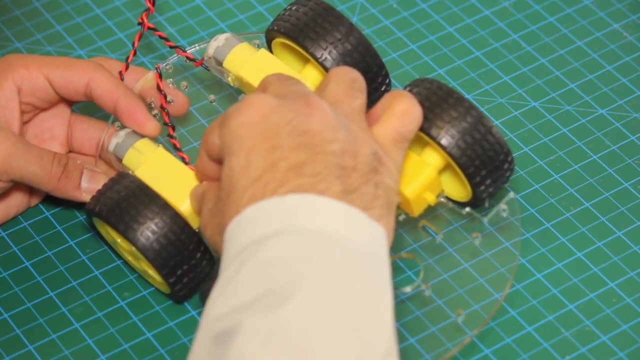 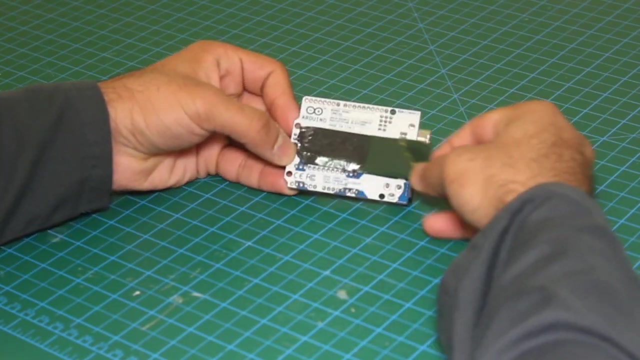 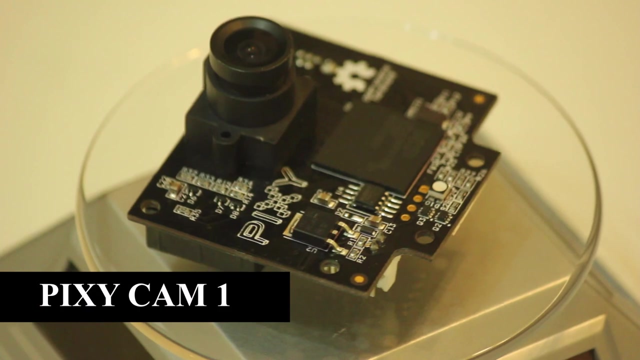 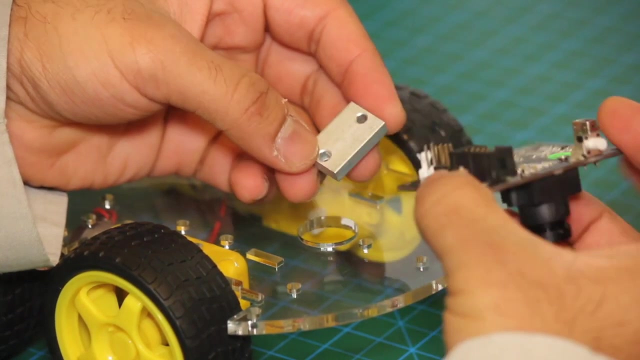 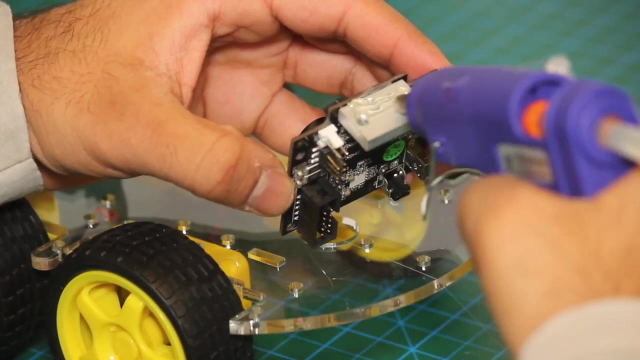 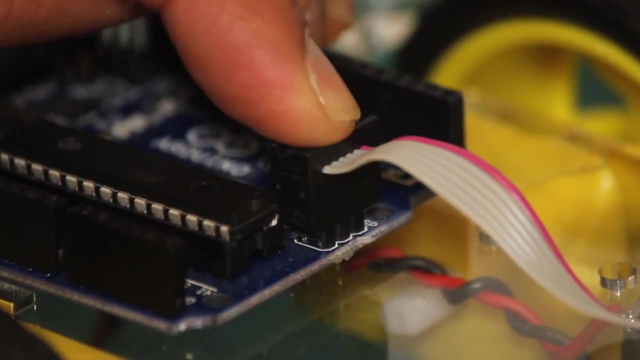 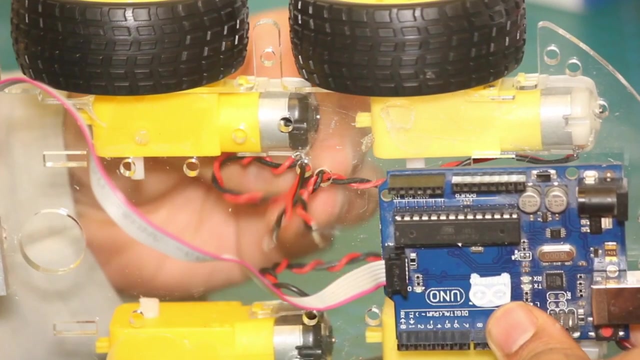 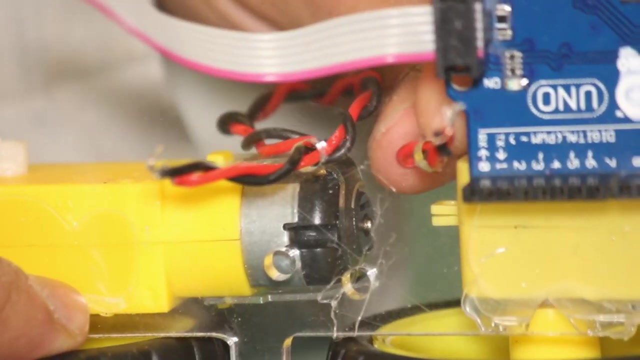 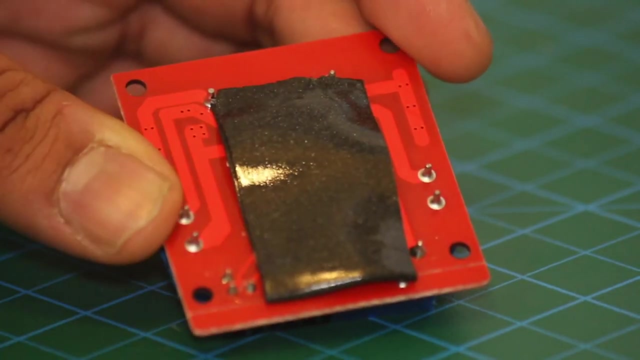 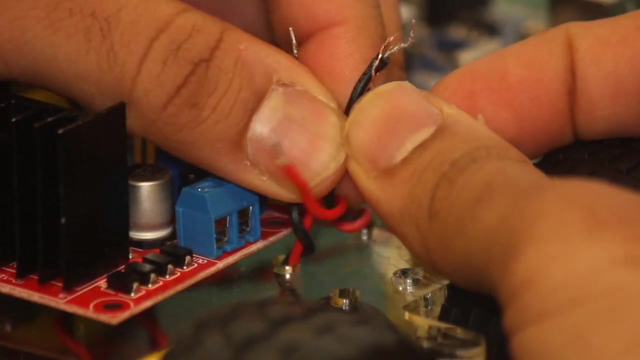 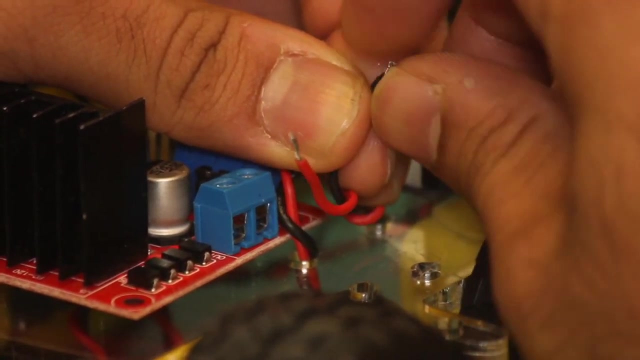 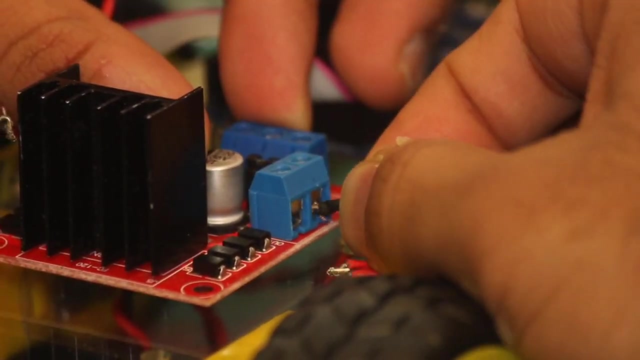 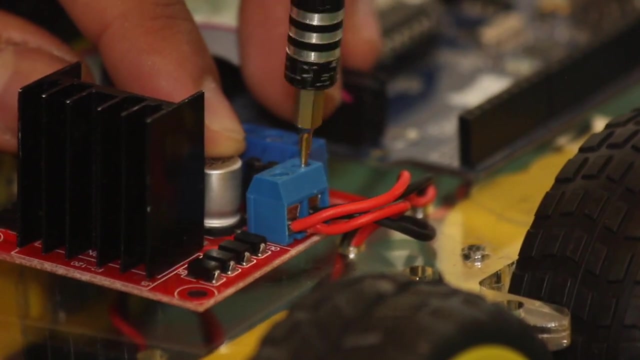 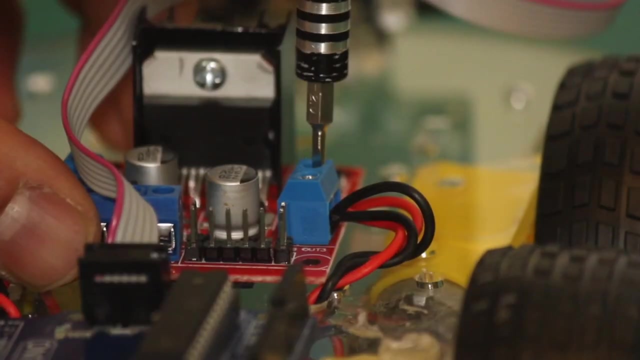 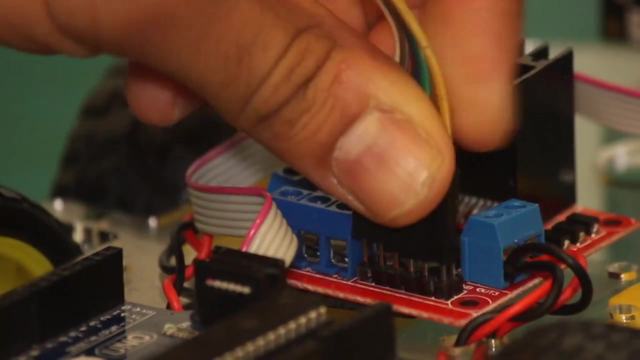 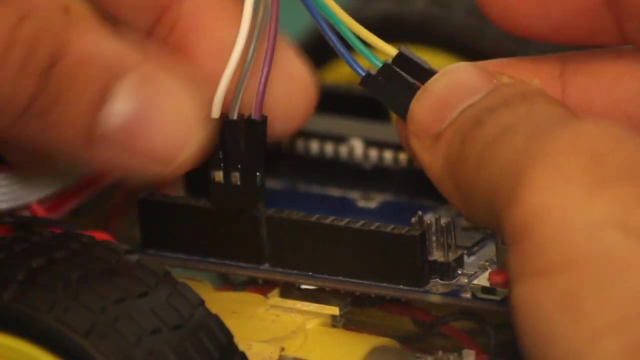 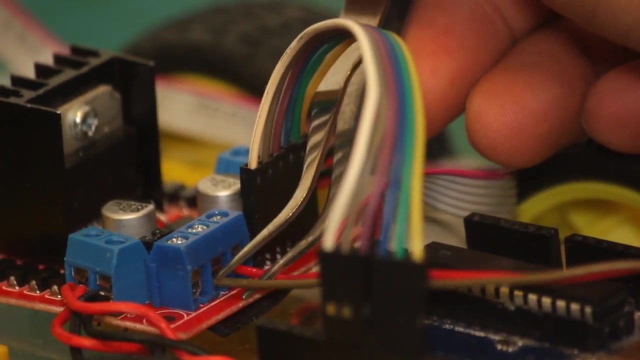 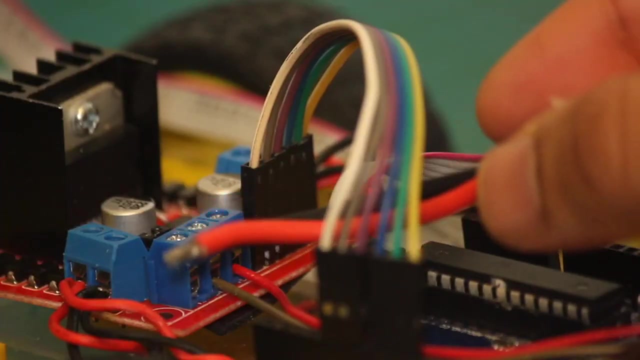 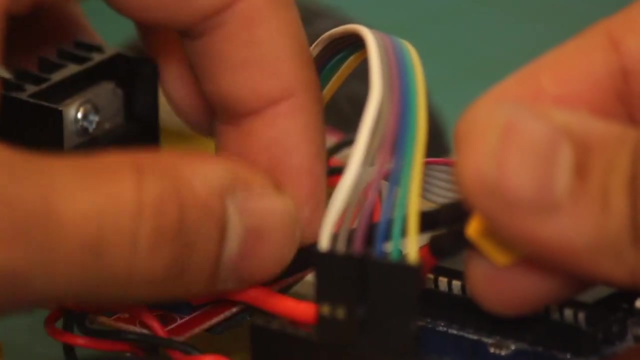 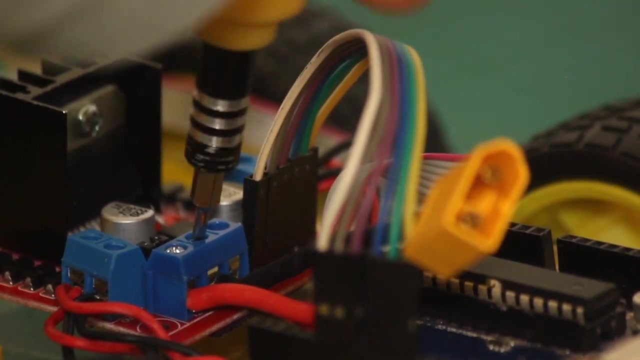 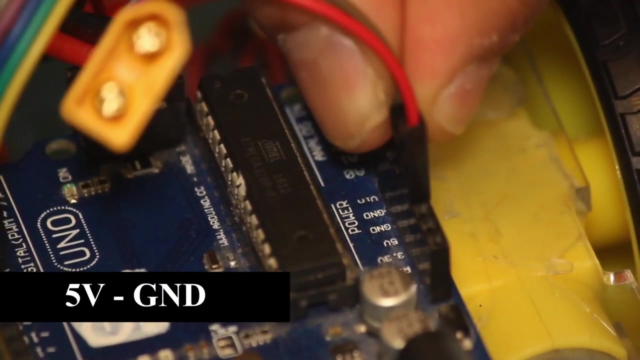 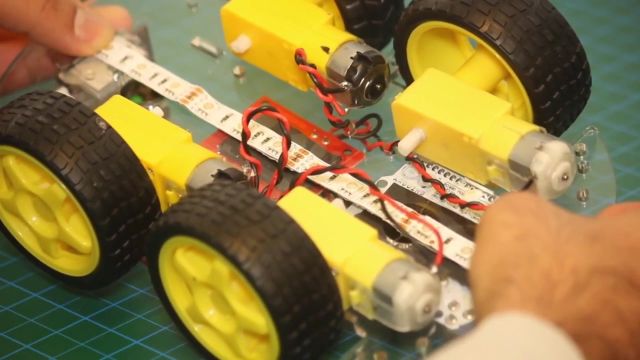 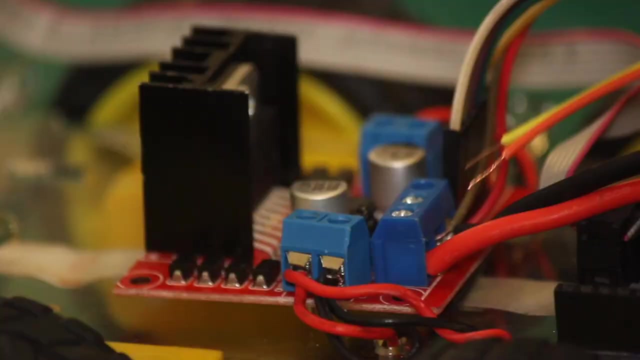 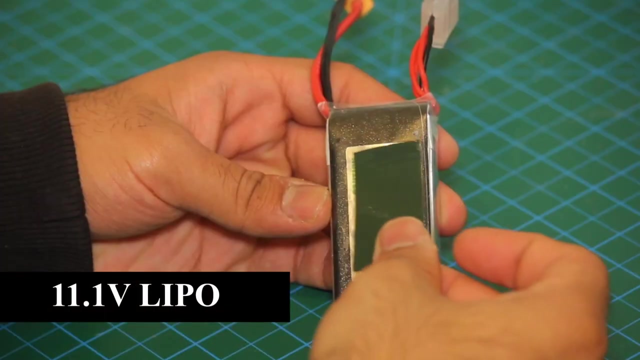 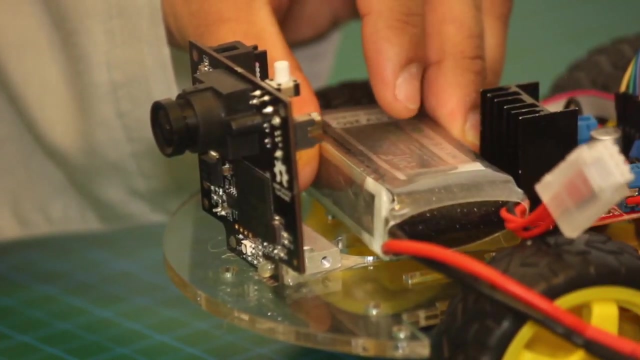 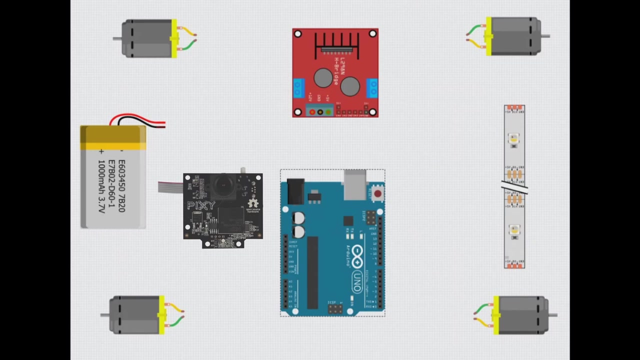 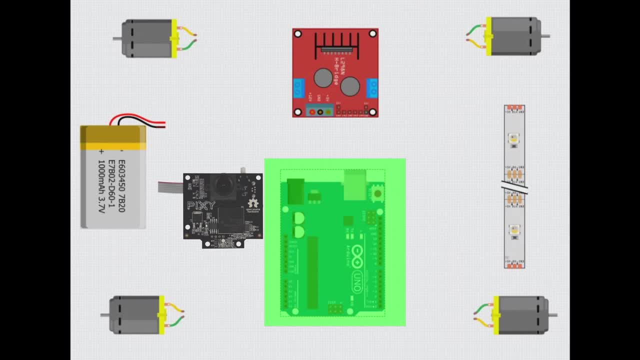 We have the Arduino board that makes all the decisions. Then we have the motor driver that lets us control the motors. We also have four DC motors, a three cell lipo battery and 12 volt LED strip For computer vision. we are using the Pixicam One. 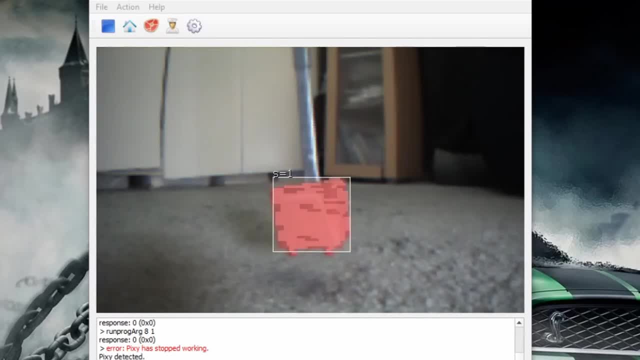 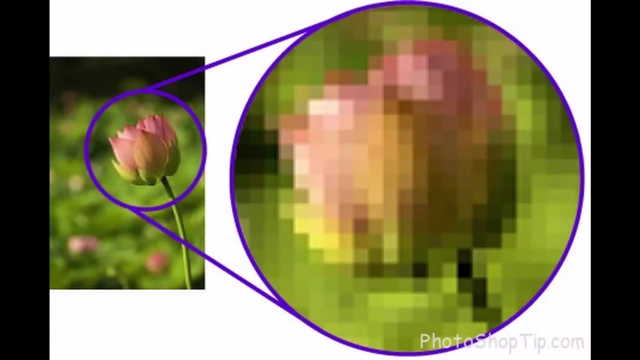 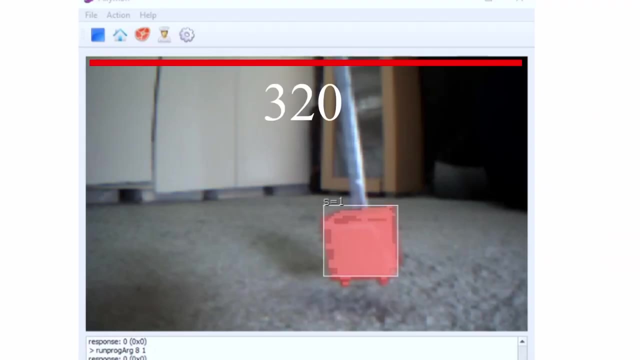 The Pixicam has a processor of its own that does all the detections and gives us the information of the location and the size of the object. So an image is just a specific number of pixels. In case of Pixicam we are getting 320 by 200 pixels. 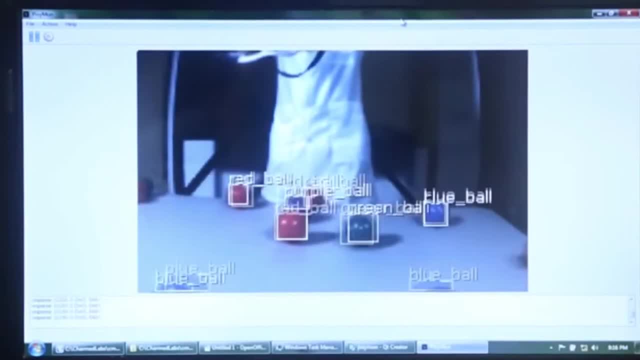 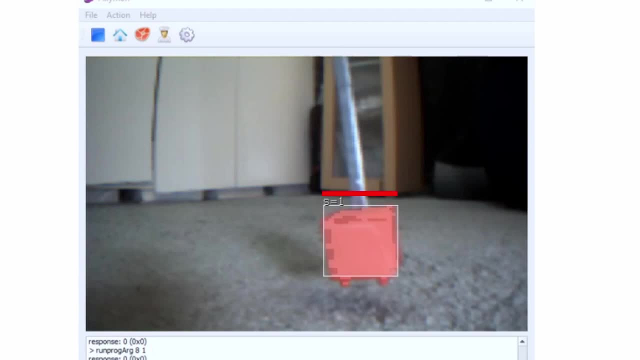 The Pixicam lets us select a colored object that we can track. The information that Pixicam sends us is the X, Y, the width and the height of the object. The X and Y are the starting points of the object. In our case, we take this information and find the center point of our object. 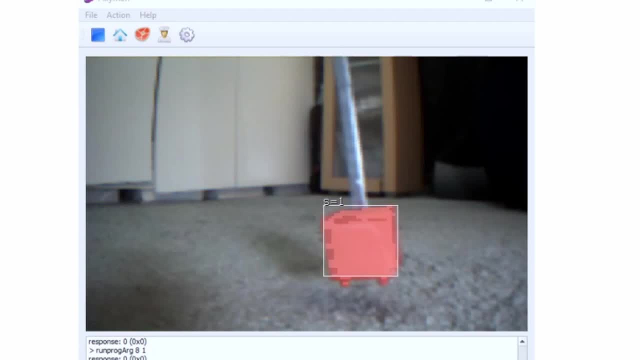 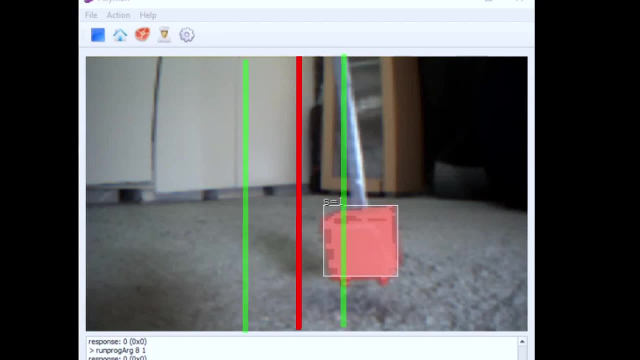 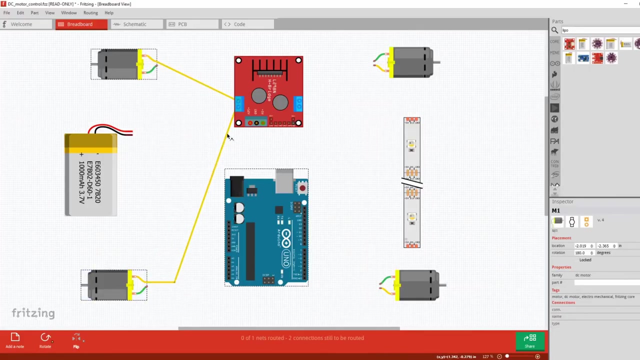 Based on this X value of the center, we determine which direction we need to move in order to come back to the center point. We also define a dead zone where the robot will not rotate, in order to avoid a lot of shaking. So first we are going to connect our motors to the H-bridge. 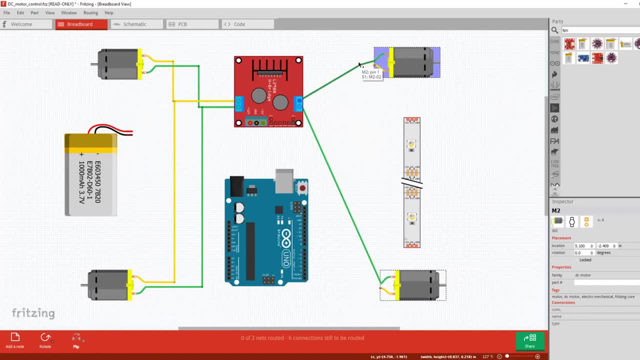 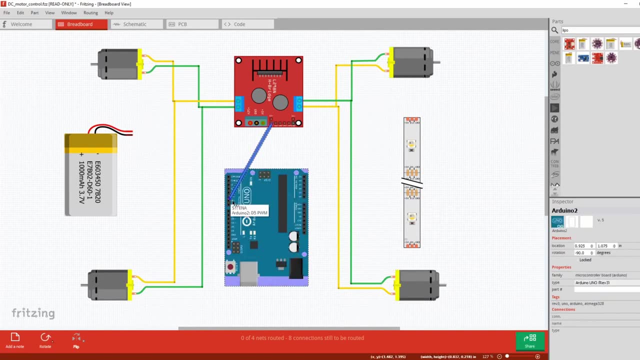 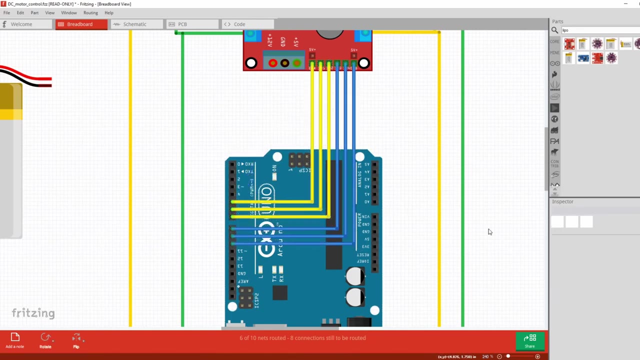 So two motors on the left hand side will be joined together and connected to the H-bridge And the two motors on the right hand side will also be connected together and connected to the H-bridge. Then we are going to connect our pins that will control the direction and the speed of the motors through the H-bridge. 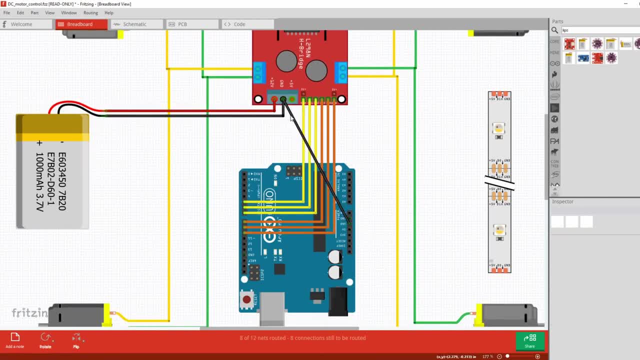 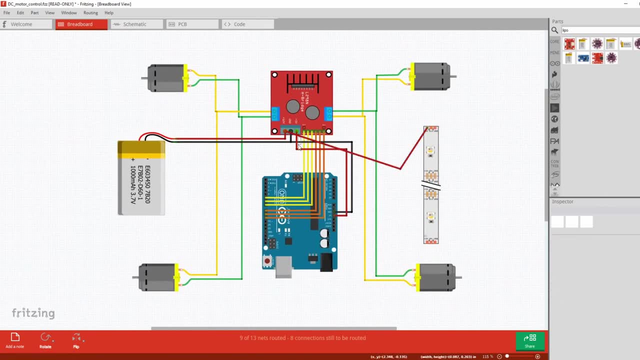 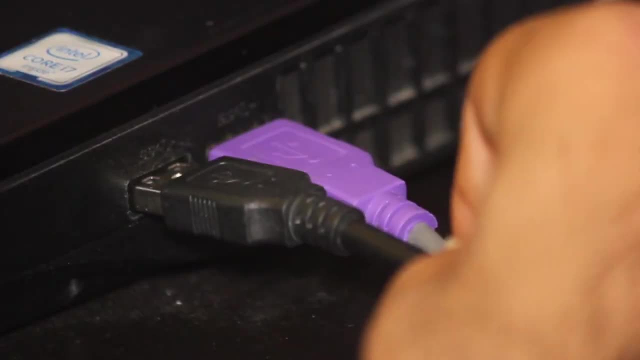 Then we will connect our battery and we are going to connect the grounds of Arduino and the battery together. And, lastly, we are going to connect our LED strip- the positive and the negative, to our power supply. Once all the connections are done, we will plug in the Pixicam. 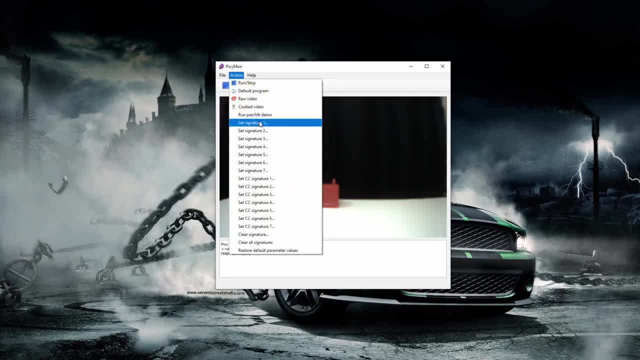 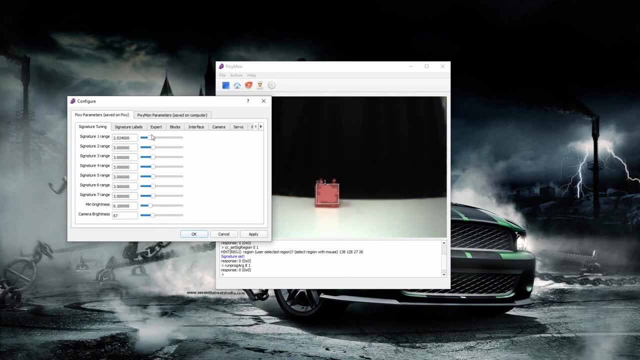 and open up PixiMoon. Here we will select our object as signature 1 and adjust the threshold value to get the optimum results. It's a good idea to add a minimum object size to avoid detecting noise. So finally, let's look at the code. 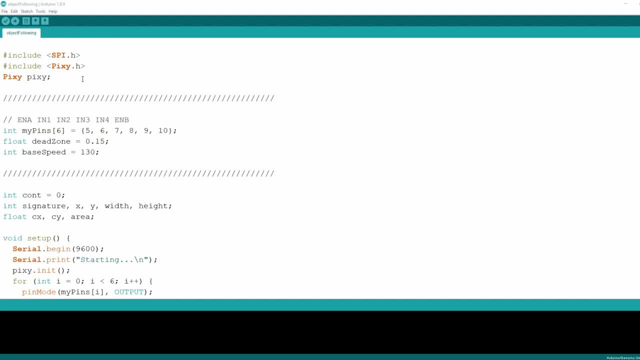 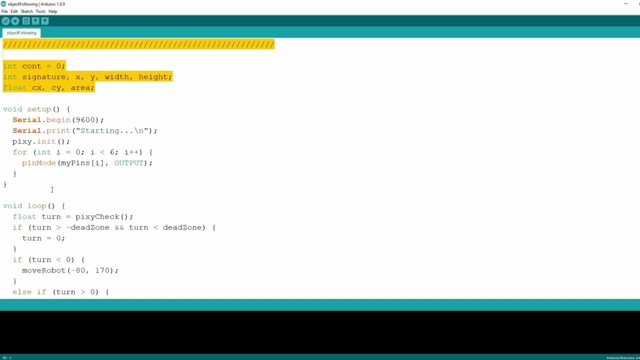 The code is actually fairly simple. We are importing our libraries, We are declaring our variables. So if you are new to Arduino, there are three main sections to the Arduino code. We have our initializations and declarations at the top And then we have the void setup and void loop. 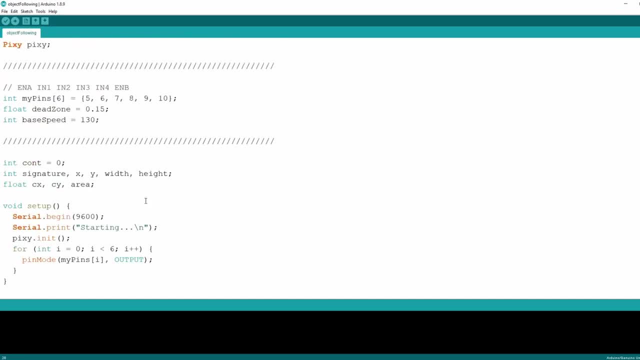 The void setup will run only once and the void loop will run continuously. So in our declarations we are declaring that our motor controller is connected to pins 5,, 6,, 7,, 8,, 9 and 10. And each of them represent their particular order. 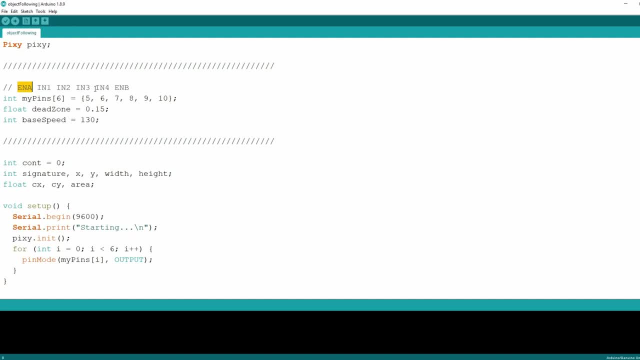 which is enable, integer input, Input 3,, input 4 and enable. So, as we discussed before, we have a dead zone that we are defining, where the object will not move at all, Which is 0.15, which means 15%, And we have a base speed at which the robot will run. 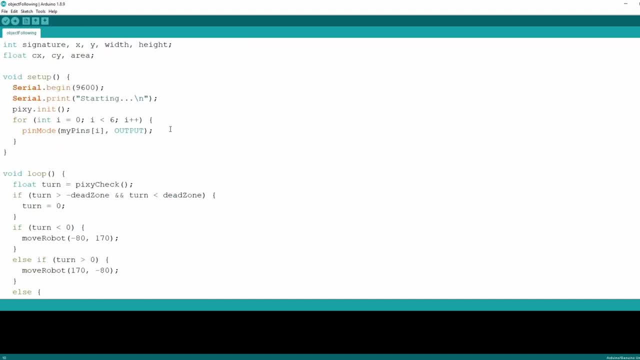 So in the void setup we are just declaring all of our pins as output using a for loop, And in the void loop we are checking the value of the turn, How much deviation we have from the center, using the pixie check function, And then we are applying our dead zone to it. 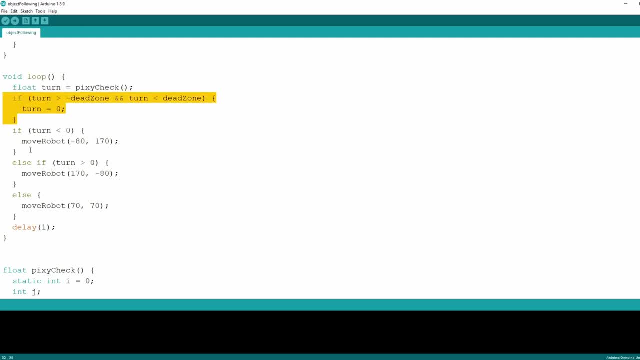 And then we are deciding how much to move the motor. So now this is a very simple code where you are just looking at if the turn is positive or negative And based on that you are moving. Otherwise you will keep going forward. Now, if you look at the pixie check function, 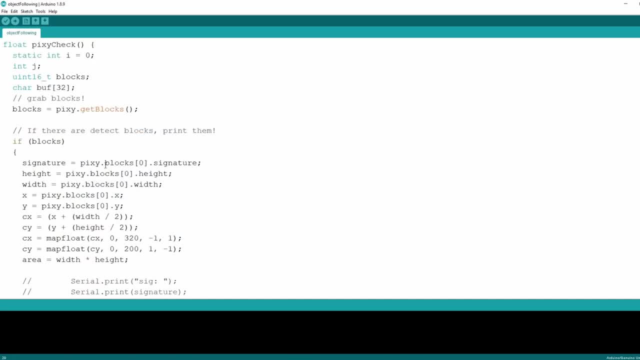 It is fairly simple. You are getting, if you are detecting any object, You are getting the x- y values of it, And then you are also getting the height and the width of it And, based on that, you are getting the center x and the center y position, as we discussed earlier. 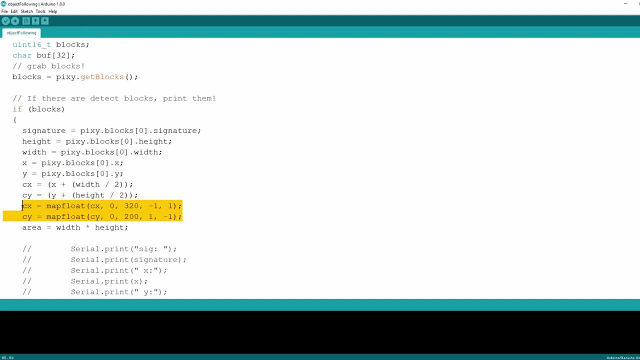 Now we are also applying normalization to it, Which means if our value is from 0 to 320. We are changing it from minus 1 to 1.. This is a common practice in the computer vision world, That we are normalizing our values.